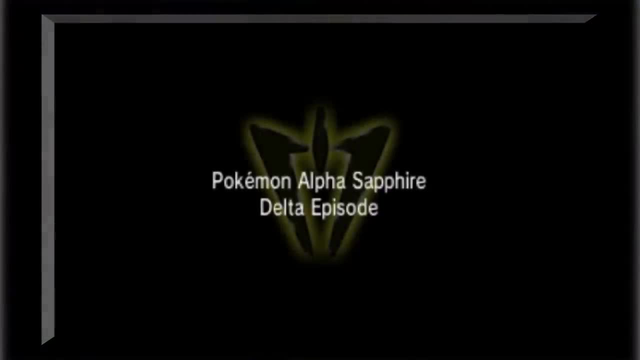 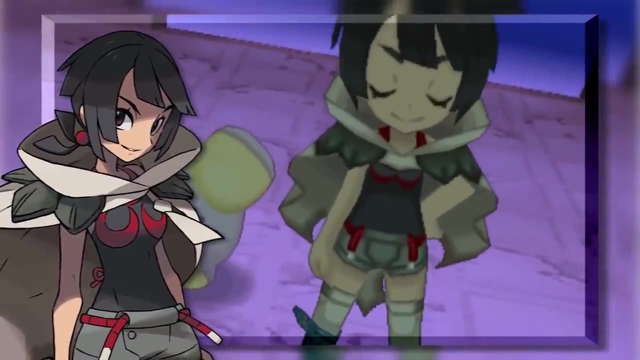 So this earth-shattering bit of post-game content is known as the Delta episode, And be wary as there be spoilers ahead. Basically, you team up with an all-new trainer named Zinnia, last in her line of ancient Pokemon, dragon worshippers. 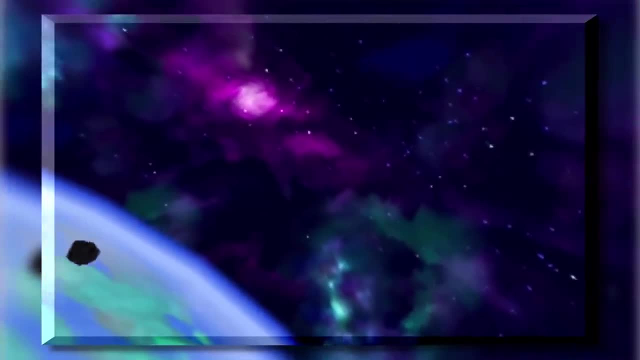 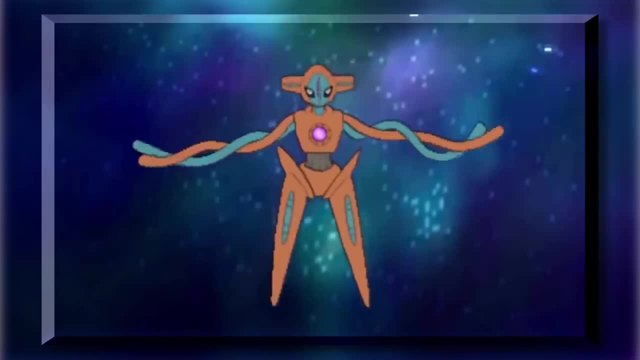 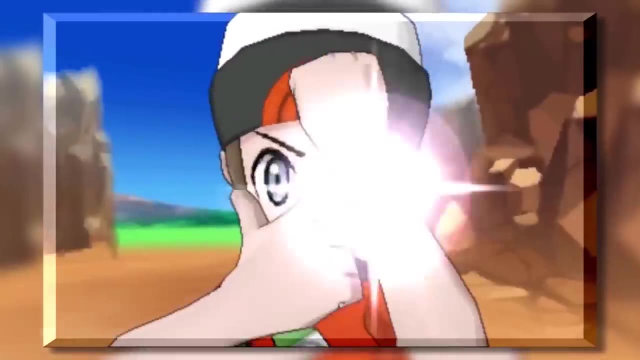 Along the way, you encounter the mysterious alien Pokemon Deoxys and the all-new mega-evolved form of Rayquaza. And yes, for those of you not keeping up with the series, there are now Mega Evolutions which are powered by the bond between trainer and Pokemon. 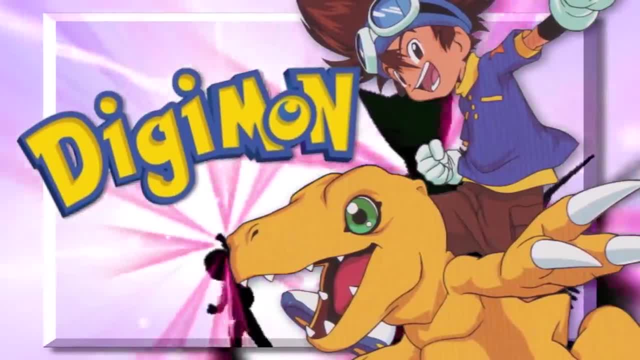 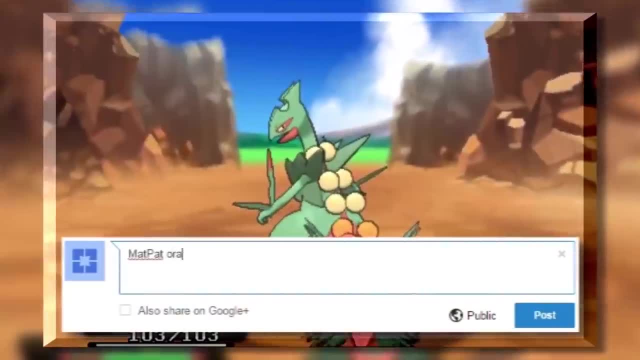 And if you're thinking that sounds a lot like Digimon, then you're thinking something everyone else realized back in 1999.. But here's why I'm doing my eighth video on the franchise, outside of the fact that you guys requested it. 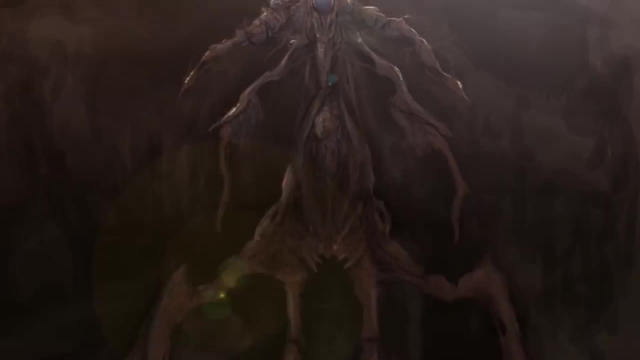 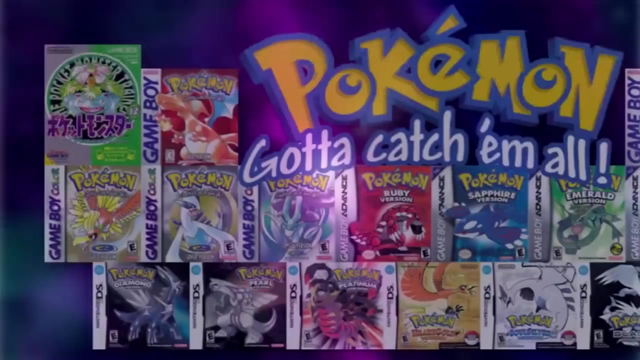 I believe the Delta episode has given us a key to finally answering some of your longest-held questions about the series, and also gives rise to a whole new line of questions regarding the nature of the two different versions of each generation. You know red and blue, gold and silver, ruby and sapphire, and so on. 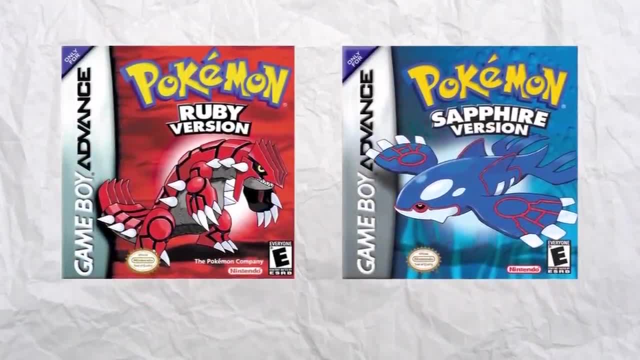 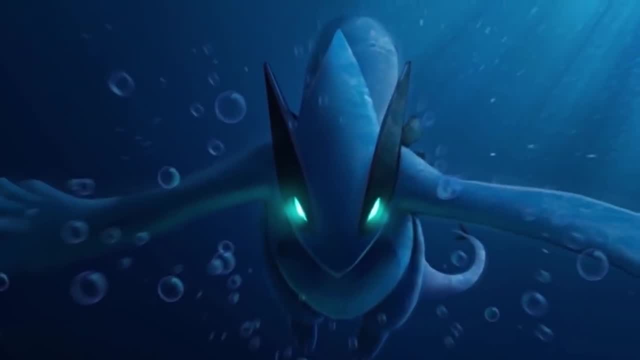 What if it's not just a ploy to convince you to buy two games when you should only really need to buy one? Well, obviously it is a ploy to get you to buy two games, but I'm talking about from a lore perspective here. 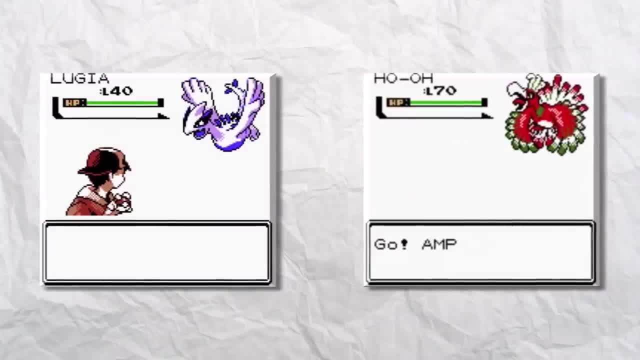 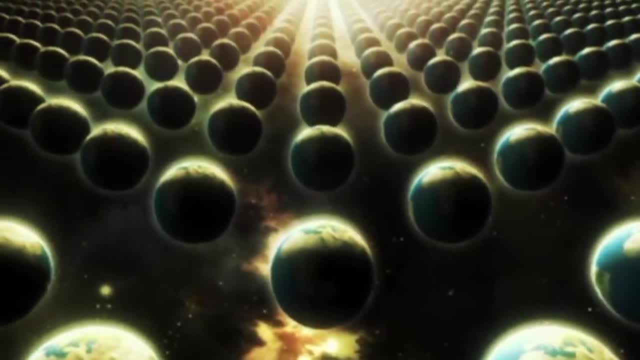 What if there's an in-game reason? the two versions are similar, yet different. Hold on to your Pokeballs. Hold on to your Pokeballs, Roma lady, because these games are set in different dimensions. You didn't mishear me. I said dimensions as in different planes of existence. 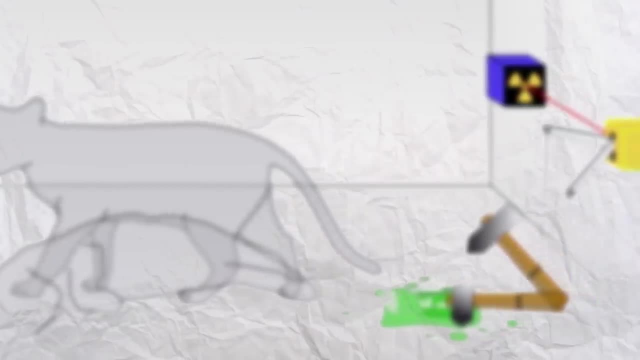 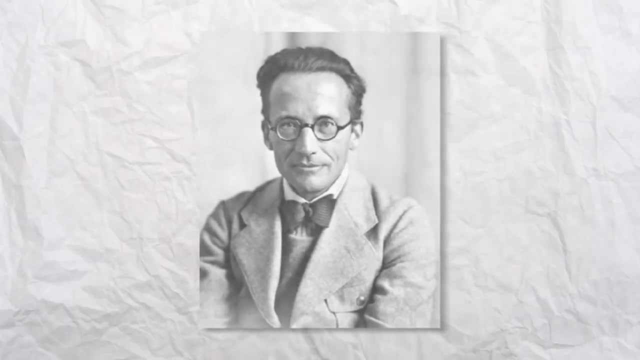 Let me explain. Normally, when people talk about these sorts of complex concepts, they start with a cat and a man named Schrodinger. But since it's Omega, Ruby and Alpha Sapphire season, let's replace this boring old Austrian physicist with one-time Pokemon champion and all-around cool guy. 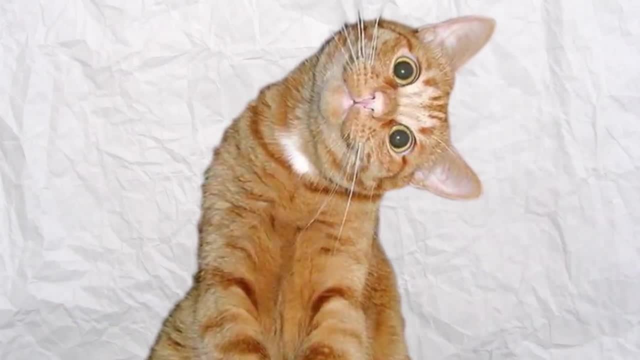 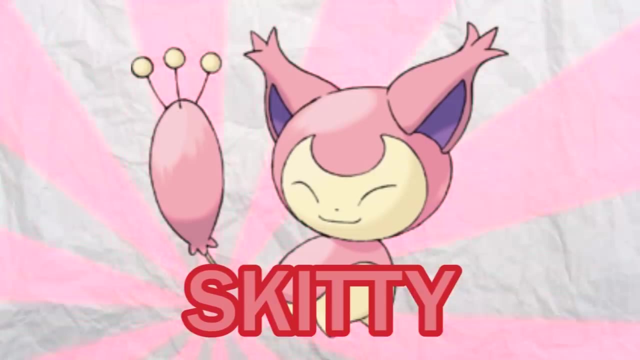 Steven Stone, And instead of a lame, non-powered cat, let's replace it with this cat-like Pokemon Skitty. Wait a minute. Skitty Like kitty, but with an S in front, And it's a cat. Oh my gosh. 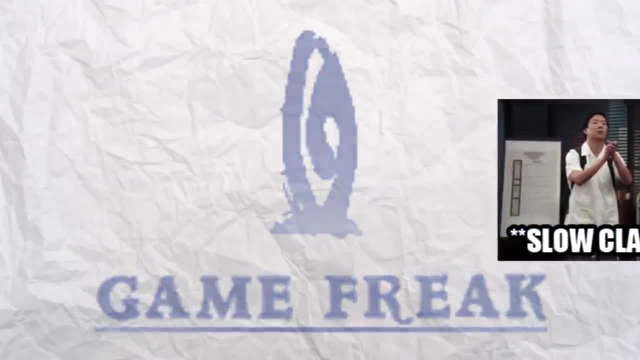 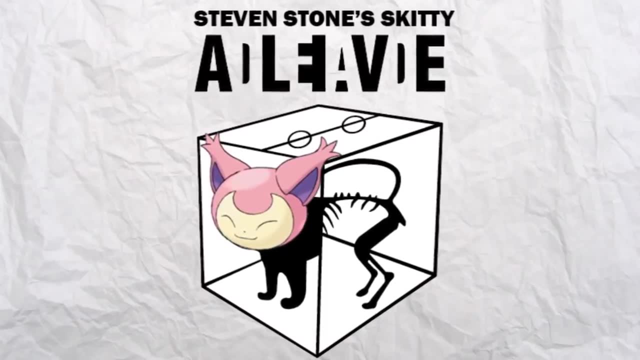 Well played Game Freak, Well played. Anyway, let's talk about the classic quantum physics thought experiment: Steven Stone Skitty. Try saying that one three times fast. It's time to get metaphysical. First, imagine that Steven Stone is standing there in the Pokemon stadium. 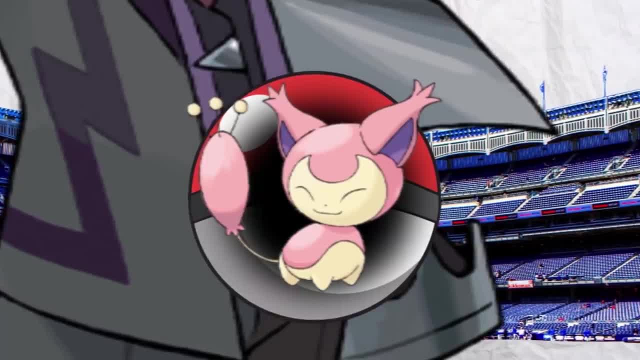 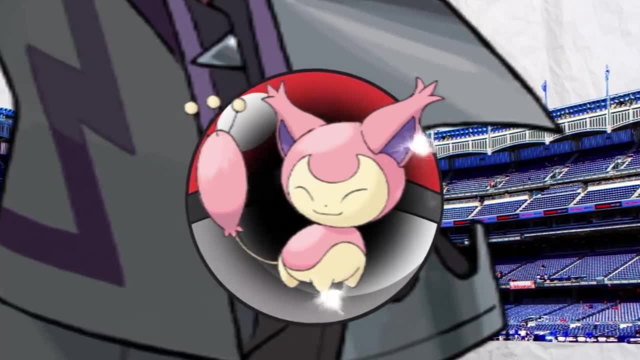 and that his weird little Skitty is just sitting there inside a Pokeball on his belt. Next, imagine that, unbeknownst to both of them, the Pokeball Skitty that Skitty's sitting in has faulty wiring, which could possibly result in the Skitty being dead. 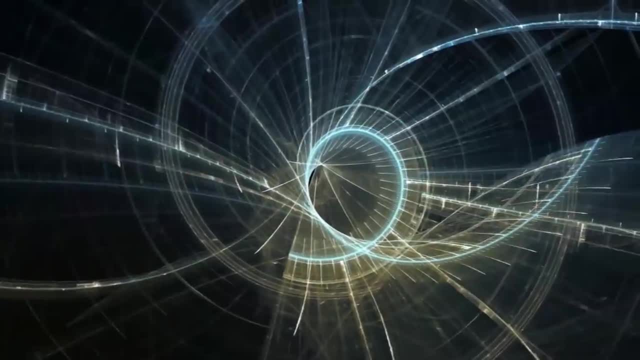 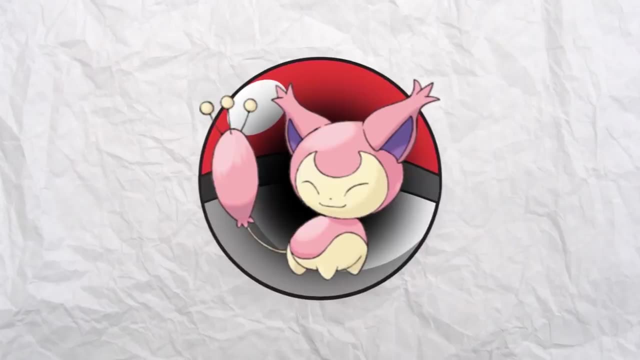 Aw, poor little guy. Now this is where it starts to get weird, because quantum physics is just bizarre. Imagine that, while Skitty lies unobserved within the Pokeball, that actually means he's in a super state of being both alive and dead at the same time. 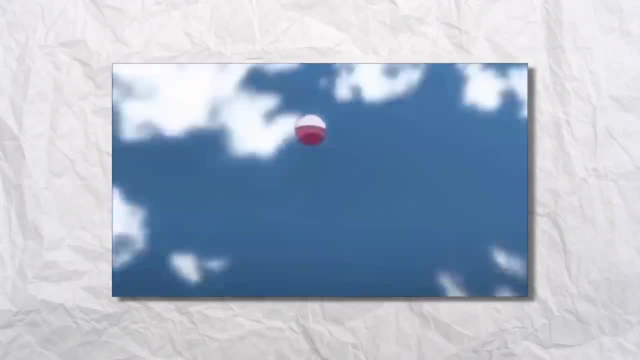 Because we don't know which he is. until the moment Steven Stone says I choose you, the Pokeball opens and we get our answer to the question. Now you quantum physicists in the room might be asking yourself: how can Skitty? 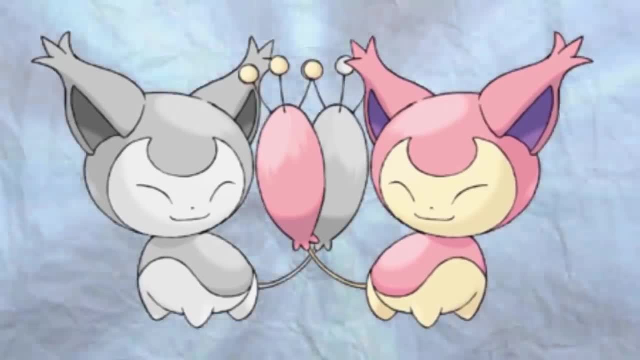 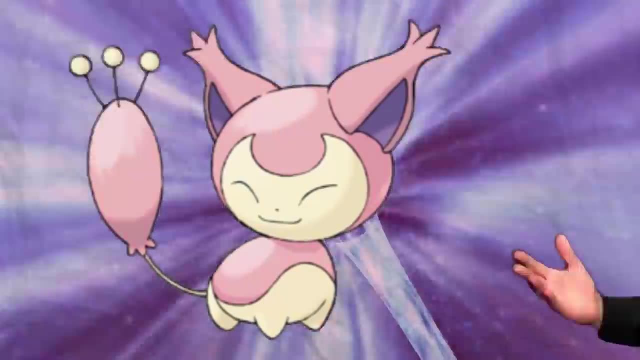 possibly be in two states at once, And then how can they collapse into one, And what determines which one he assumes? Well, my little would-be Pokemon masters. the truth is no one really knows for sure, But there are a few commonly discussed theories. 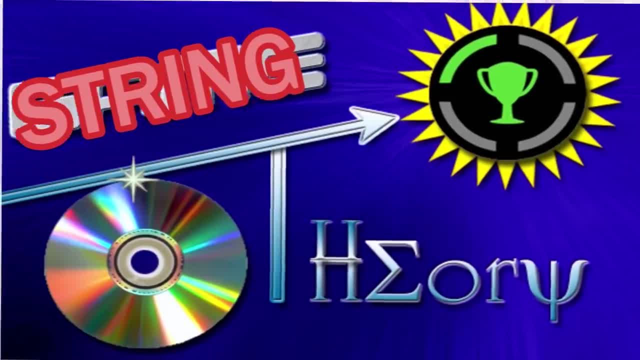 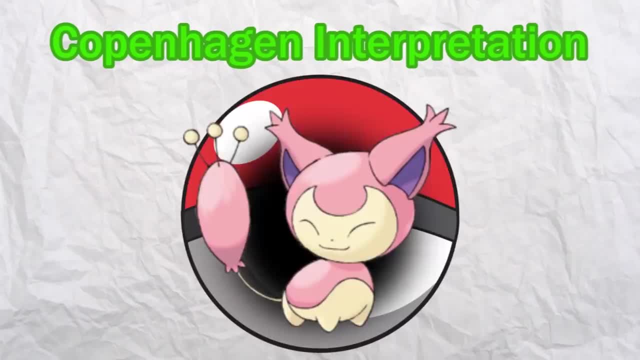 string theories. thanks for observing No Little science joke. Ah, whatever, The theory we just discussed is called the Copenhagen Interpretation, that in observing the Skitty we collapse. the two possible outcomes to one true outcome, Skitty being either. 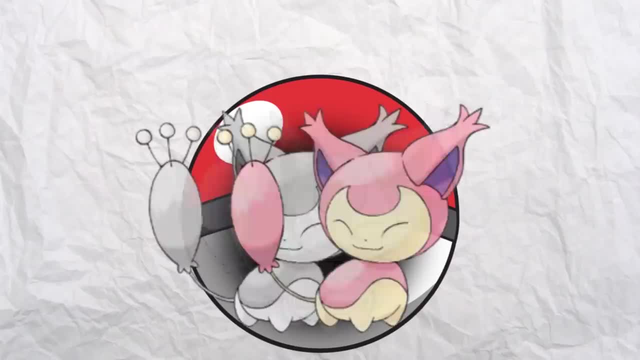 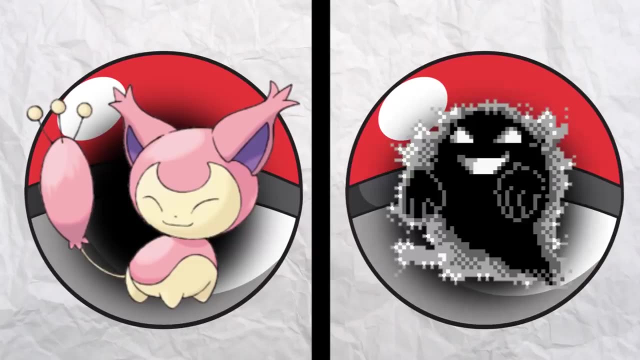 alive or dead. But another theory is that that collapse never happens, That there is a universe for each possibility: One where Skitty pops out and is alive and another where it's sadly a bit more than fainted. This is known as the Many Worlds Interpretation. 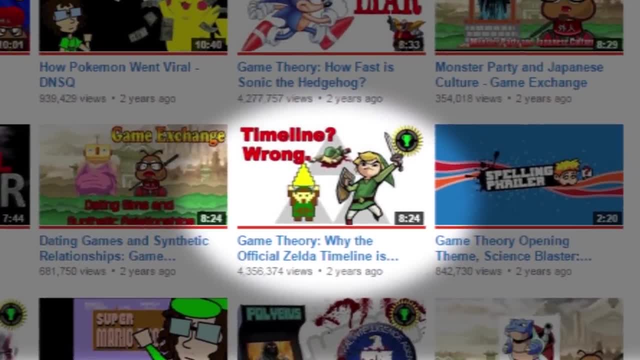 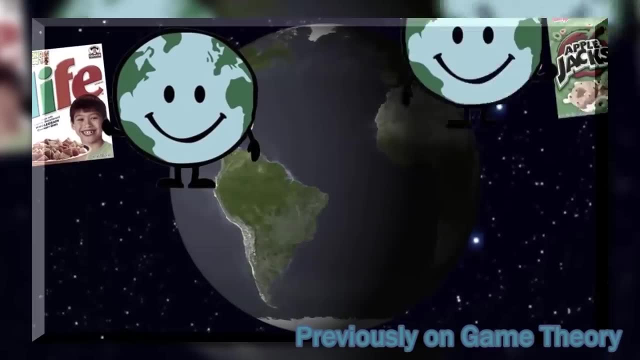 And if you're a true loyal theorist, you might remember this episode. I did yikes a little over two years ago About how the Zelda timeline is wrong, Where I explained that every situation with multiple outcomes creates an entirely new parallel universe. 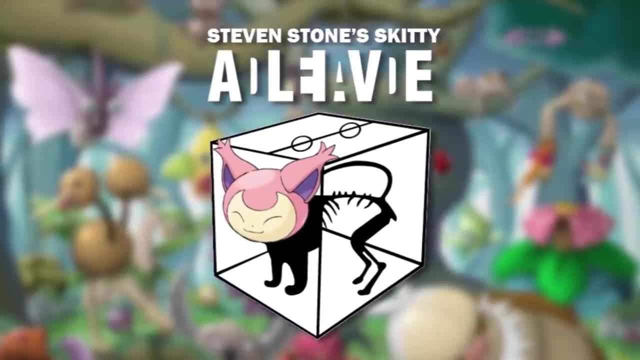 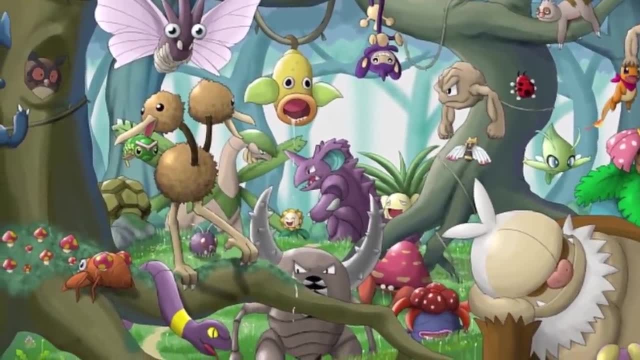 Well, that's one thing. That's one way to explain Steven Stone's Skitty too. But now, instead of just one Pokemon's life hanging in the balance, imagine it was a significant percentage of the total Pokemon population on the planet. 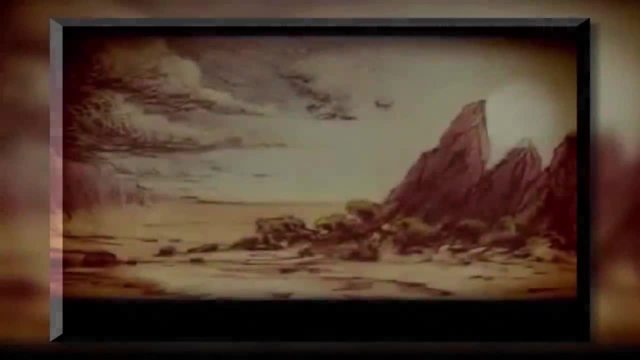 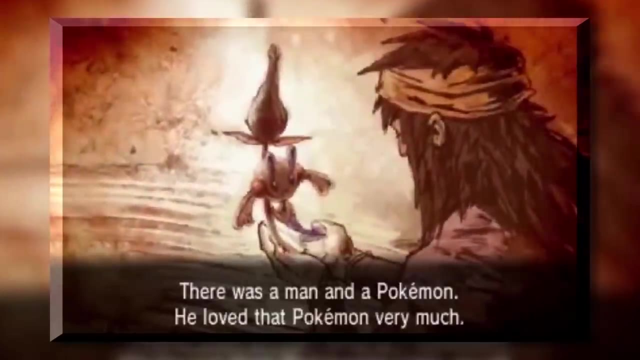 Which leads us back to the franchise's lore. According to Pokemon X and Y, 3000 years before the events of the game, there was a trainer named AZ who lived in the Kalos region with his beloved flower-bearing fairy, Pokemon Floette. 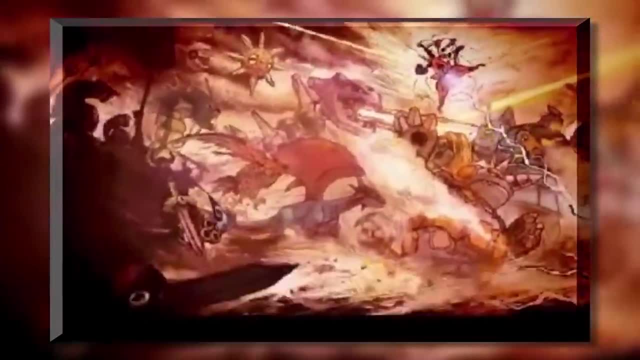 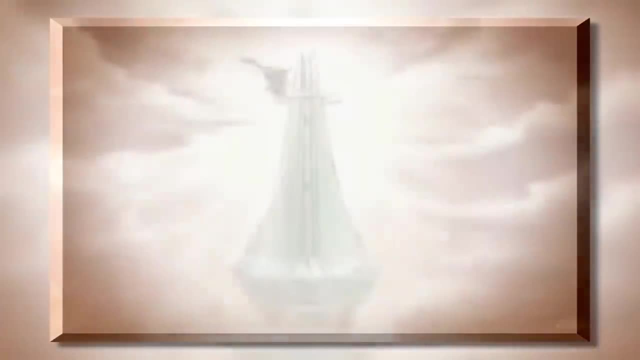 Unfortunately for both of them, a war suddenly broke out in the region and the Floette was called upon to fight. Sadly, Floette was killed in battle and AZ was devastated. AZ went crazy trying to build a machine that would bring his Floette back from the grave. 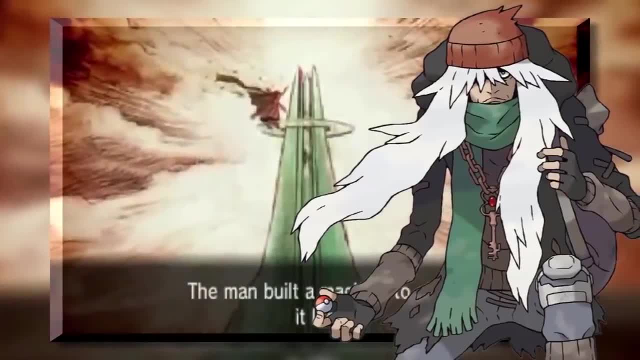 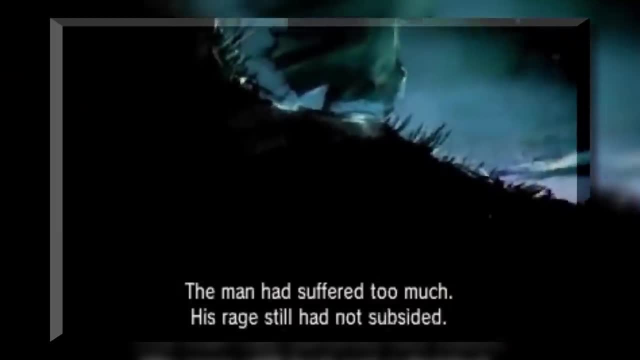 And in that process somehow developed the ability to live forever. I don't know, it's a theory for another day. What's even crazier, though, is that he eventually succeeds, But by now he's so maniacally deranged about ending the war at any cost. 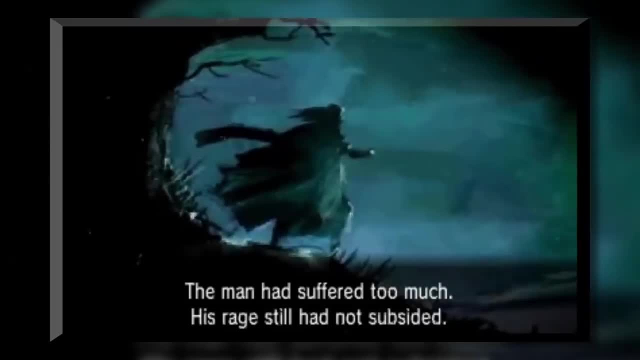 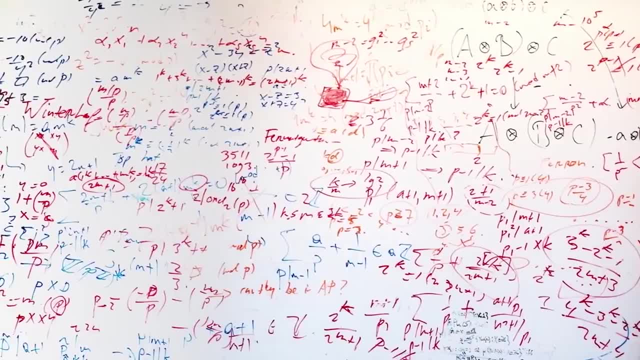 And the whole awful series of events is so urgent that it's almost impossible for him to survive. Now I would be skeptical too. I mean, this is way too complicated for a kid's game. Except that it isn't The games actually support this theory. 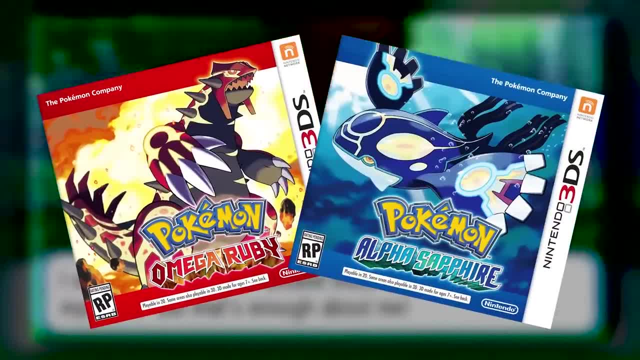 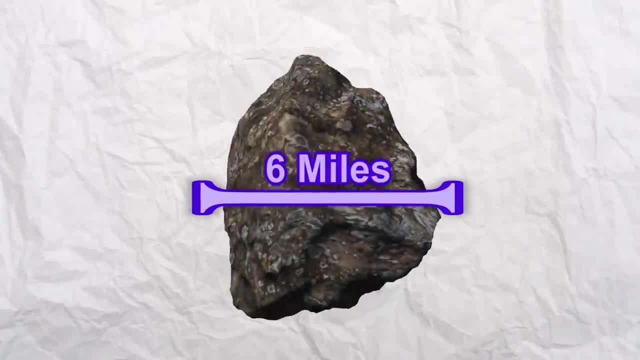 Fast forward to Omega Ruby or Alpha Sapphire during the Delta episode, In case you missed it the first time because you were still trying to figure out that super esoteric Garatina joke: an asteroid six miles across, the same size as the one that probably killed dinosaurs. 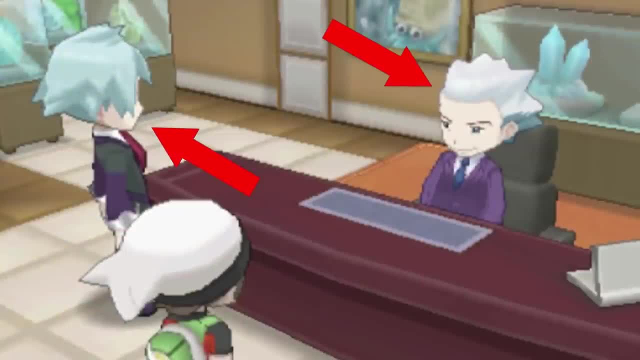 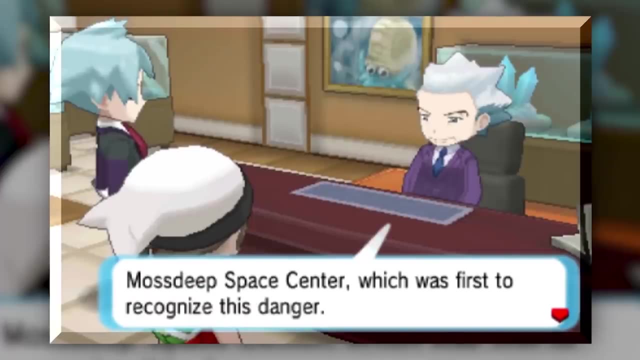 is on a collision course with Earth. Mr Stone, Steven Stone's father and head of the Devon Corporation, explains that his company has harnessed the same energy AZ created with his weapon to power many of the high-tech gadgets that appear throughout the Pokemon world. 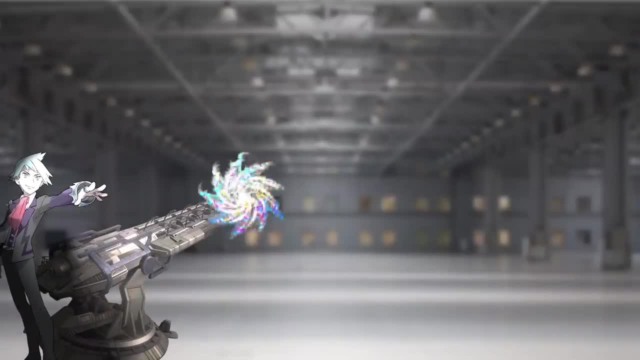 including one that's about to help you save the world by tearing a hole through reality and opening a portal to another dimension for the asteroid to fly away through. Yeah, This is uh still a game about capturing cute little pocket animals and having them slap each other around, right? 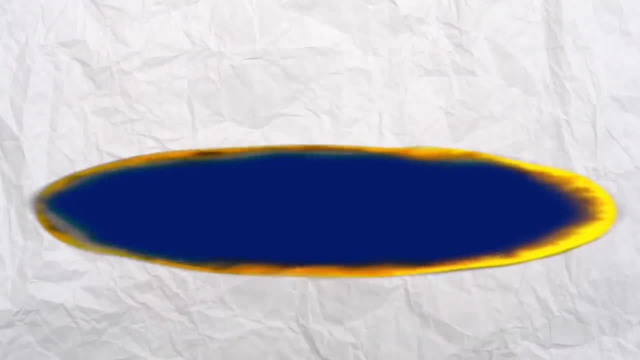 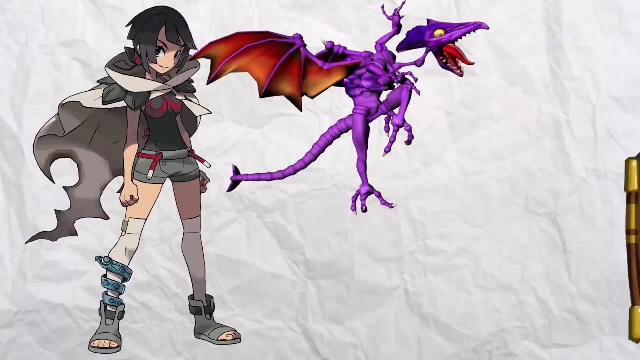 Anyway, seems like a great plan right. Rip open a dimensional rift, bada bing, bada boom. asteroid crisis over Easy squeezy, lemon peasy, Enter. Zed Zinnia, Weird dragon girl descended from Ancient Protector in the Bold or something, doesn't really matter. 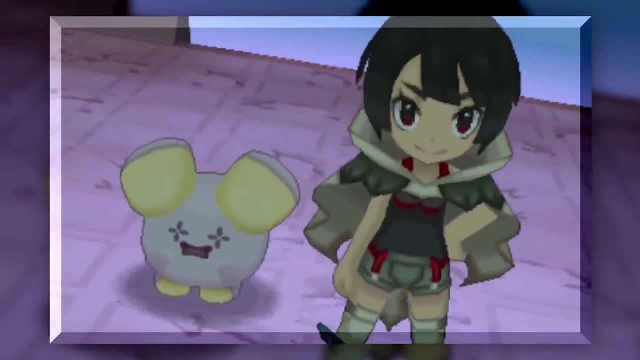 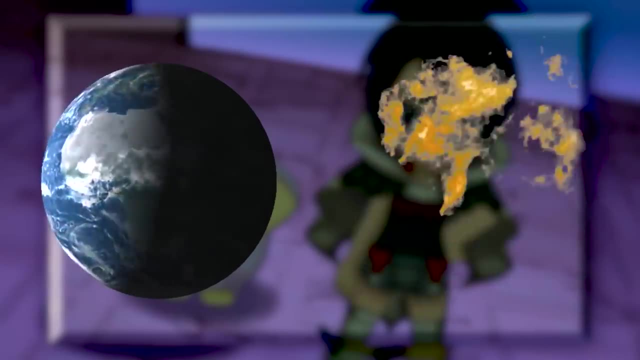 Her hidden ancient dragon knowledge warns that in this other dimension there's a planet just like yours, but different somehow, And sending the asteroid to them will just destroy their planet instead of yours. Here's some quotes. That is an impressive machine. Snap your fingers, the asteroid vanishes and we all live happily ever after. 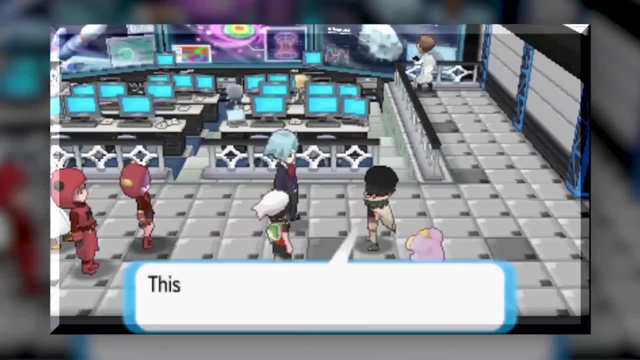 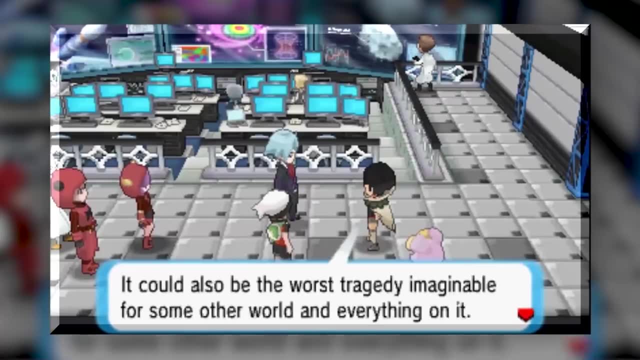 Ah, ha, ha, ha ha. Indeed, It's like that former champ said: this thing is the best hope we have of saving this planet and everything on it, But you know, it could also be the worst tragedy imaginable for some other world and everything on it. 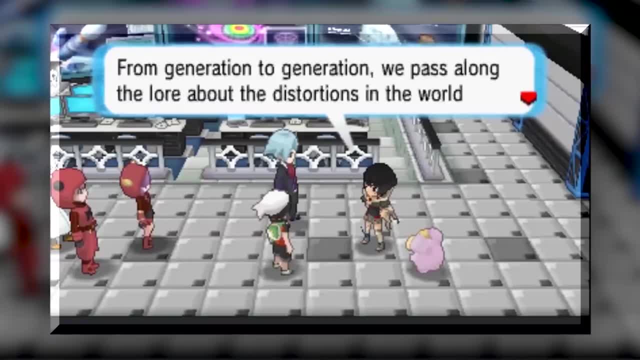 My people know it From generation to generation. we pass along the lore about the distortions in the world born by the mega evolution mechanism and about the existence of another world which we have long observed to be just like this one and yet not the same. 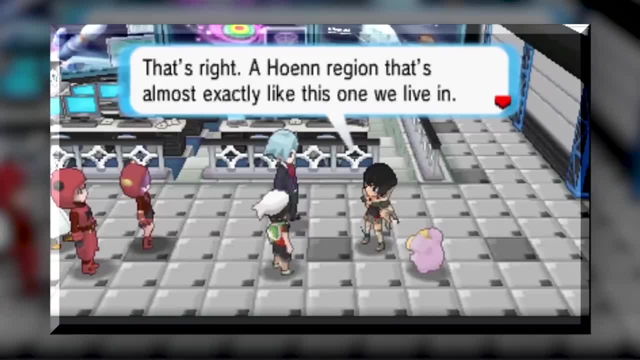 That's right. A Hoenn region that's almost exactly like this one we live in, filled with Pokemon and people like us, A world where maybe the evolution of Pokemon took a slightly different path, Where mega evolution is unknown. A world where that war 3,000 years ago never happened. 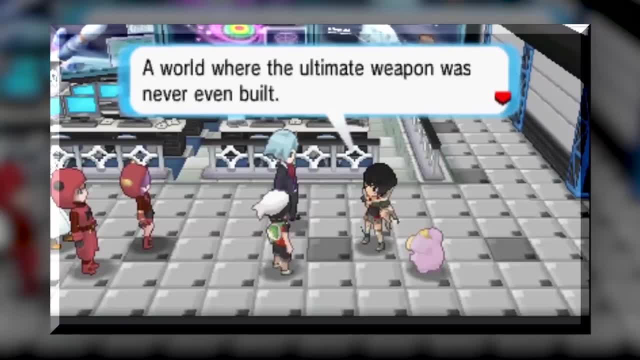 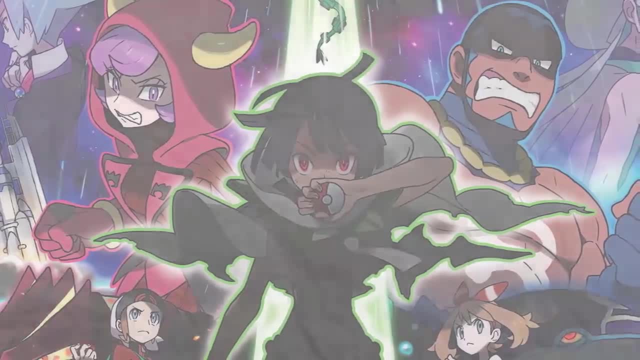 A world where the ultimate weapon was never even built. End quote. This is pretty heavy stuff. It's also stuff that seems to imply that our mega evolution theory is correct. The 3DS Pokemon games, Pokemon X and Y and Pokemon Omega, Ruby and Alpha Sapphire. 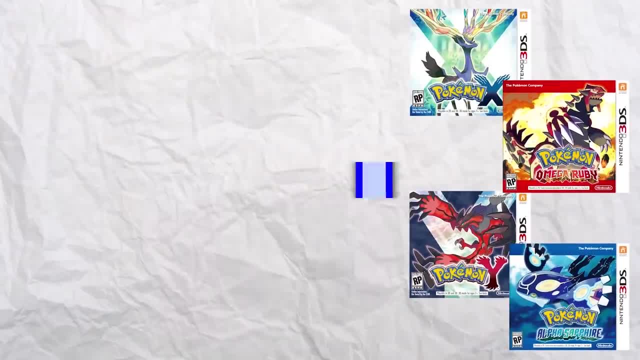 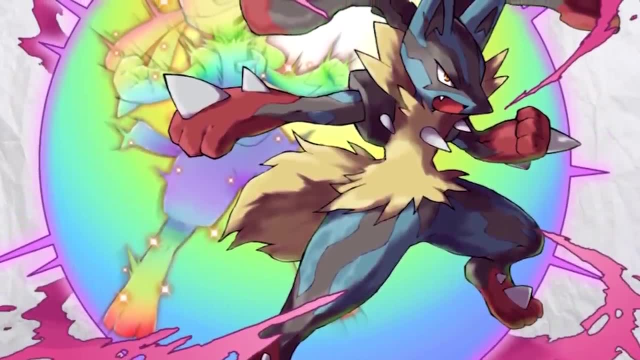 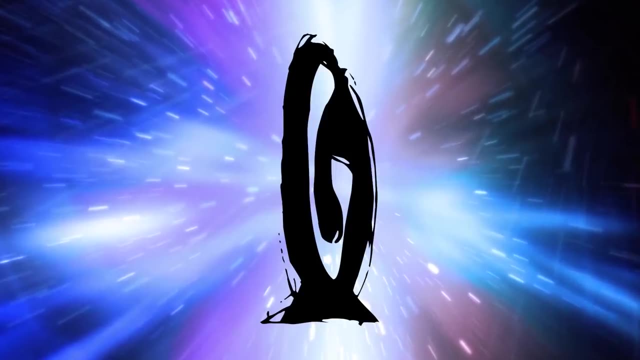 are set on a different timeline, a different dimension, than the other games in the series, Which also rather conveniently explains why mega evolution is so important. It explains why mega evolution never existed as a gameplay feature until now. Using the many worlds interpretation, Game Freak has created the ultimate retcon. 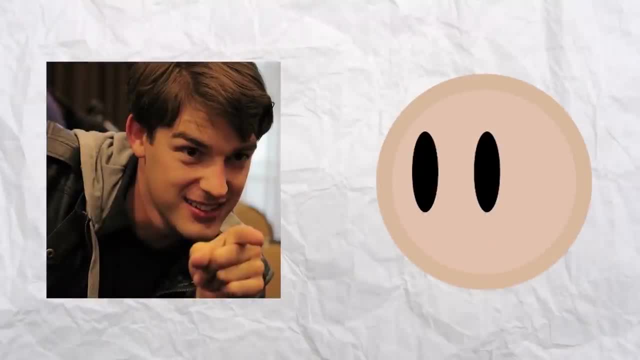 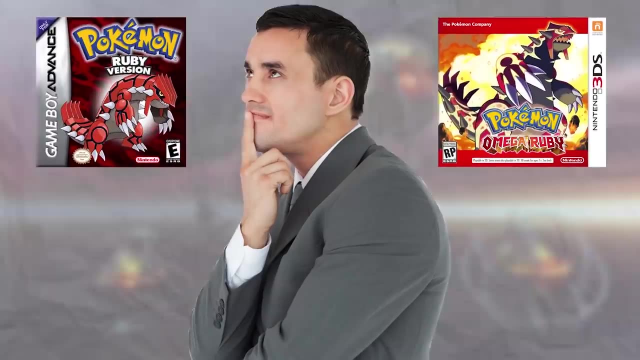 And while that's pretty impressive in its own right, I know you And I know you're still not quite satisfied, because that's not what I originally set out to prove. So how does this translate to the different versions being set in alternate dimensions? 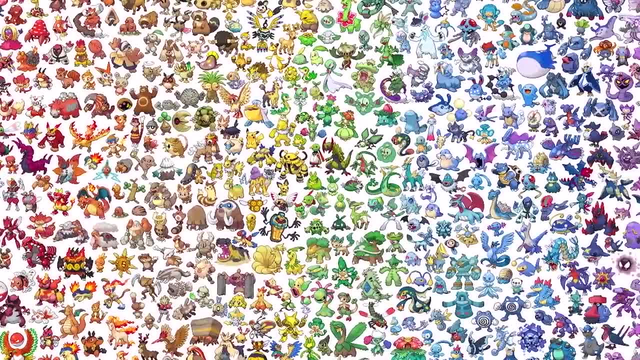 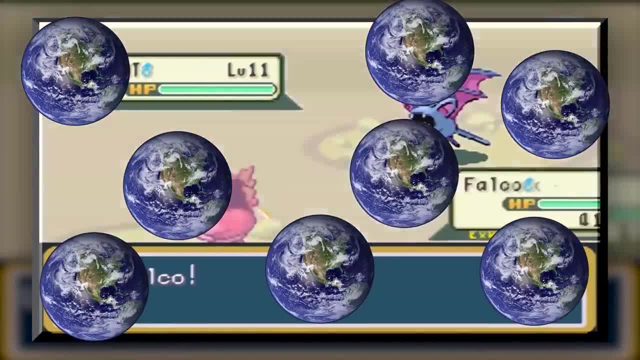 Well, look at what we've learned In the world of Pokemon. the many worlds theory seems to be a fact. Different versions of reality are definitely created Whenever events have multiple possible outcomes, Leaving a bunch of really similar universes to float around in the ether. 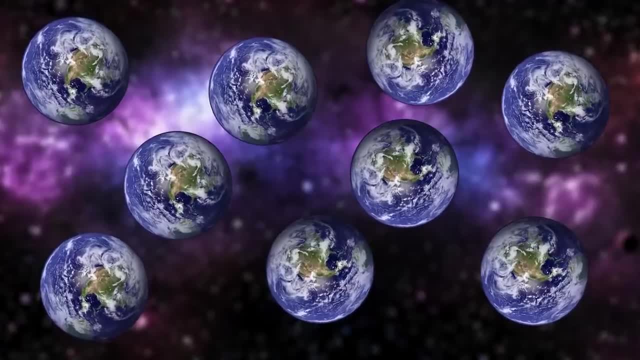 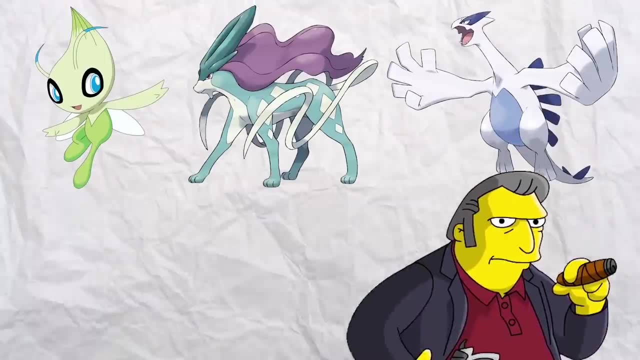 With little differences between them, Like, uh say, which Pokemon are available on any given route, Or maybe which legendary Pokemon the criminal syndicate has chosen to be a part of their master plan, Or the name of Professor Oak's human turd of a grandson. 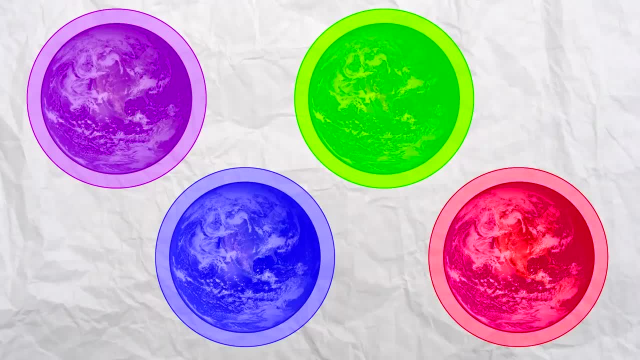 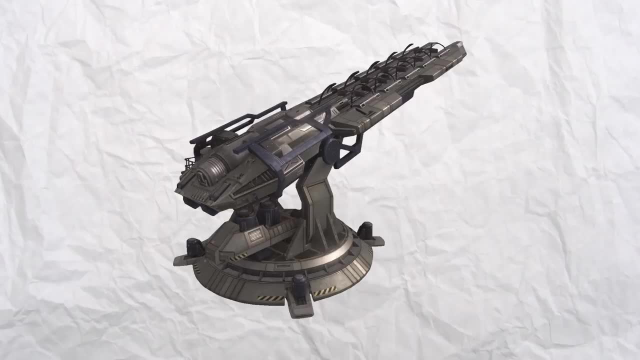 All different universes, differentiated by different titles. But we can take it one step further. That rift creating device had a name. It was called get this a link cable. And while the opening of this episode may have made me feel like Father Time, 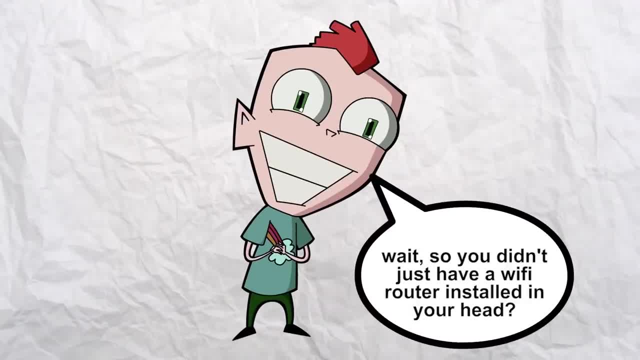 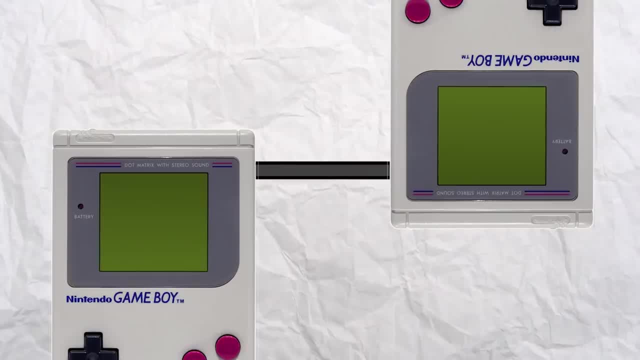 I'm sure at least some of you out there watching in the audience can remember, or at least have heard about, a time before wireless communications technology, When us Pokemon fans had to buy a device that would physically link our Game Boys together when we wanted to battle or trade. 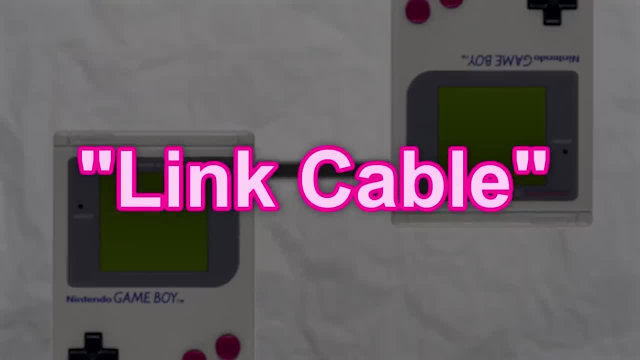 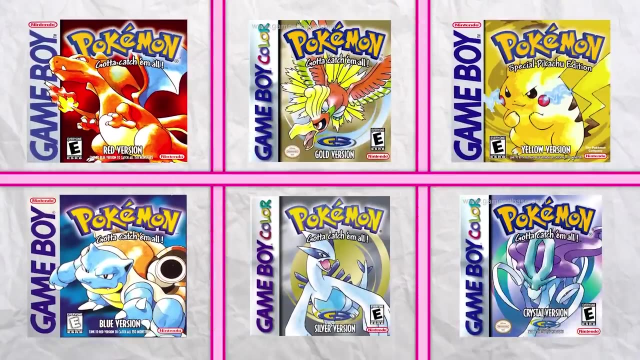 A device that was called a link cable. Why is this a big deal? Well, we can extrapolate that not only are red and blue, gold and silver and so on different talents, And that these are the feelings of the same basic story set in parallel universes. 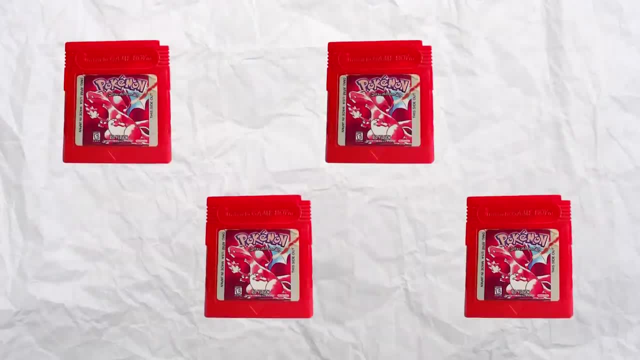 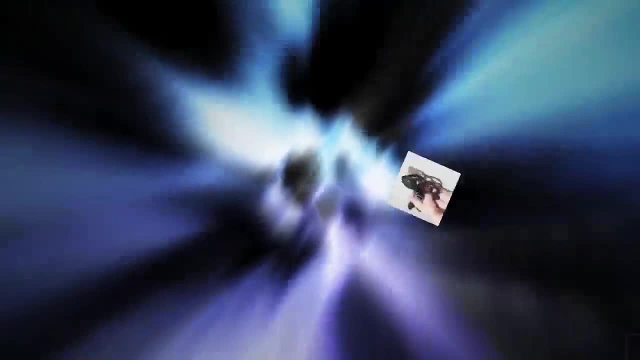 But that, in fact, each copy of each game is in fact its own universe too, And that these link cables actually physically connect them via rifts in time and space. Want to trade or battle with a friend? Well, doing that spreads new Pokemon from one dimension to the next. 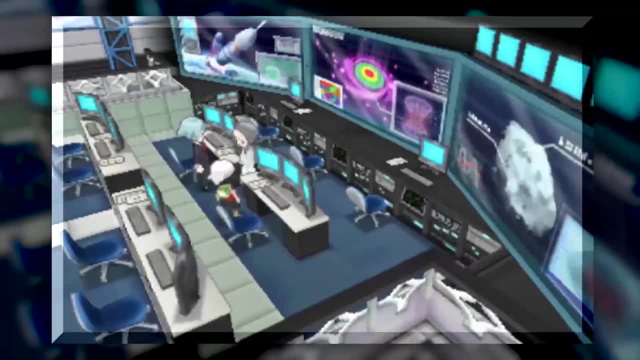 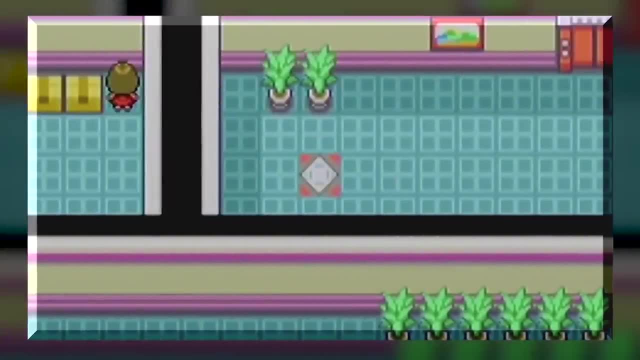 And that's not even where it ends. There's even a scientist in the game who explains that the Devon Corporation casually uses this technology all the time In devices that people use every day. He only mentions those overused warp panels, But think about all the different bizarre things this could explain. 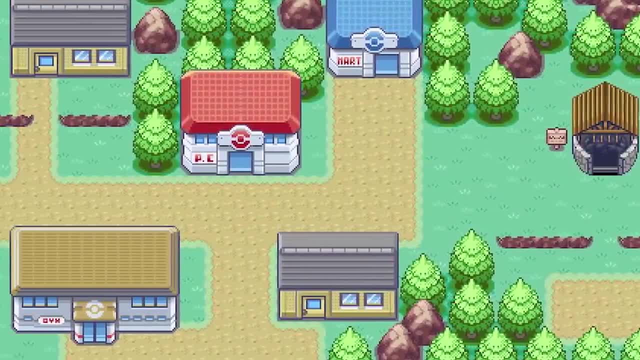 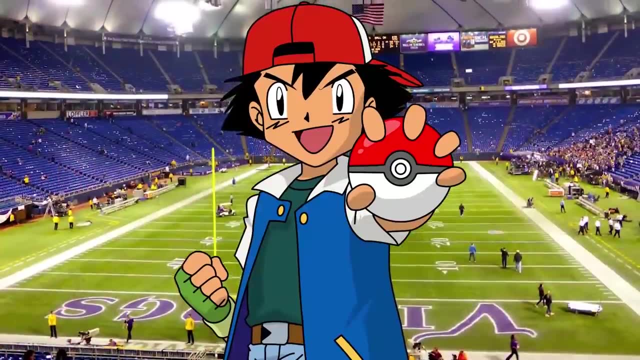 I mean, this is a civilization that can travel through any possible reality. What else could you do? Well, how about impossible references to real world pop culture, Like when Ash references the Minnesota Vikings in the Pokemon movie? I didn't know Vikings still existed. 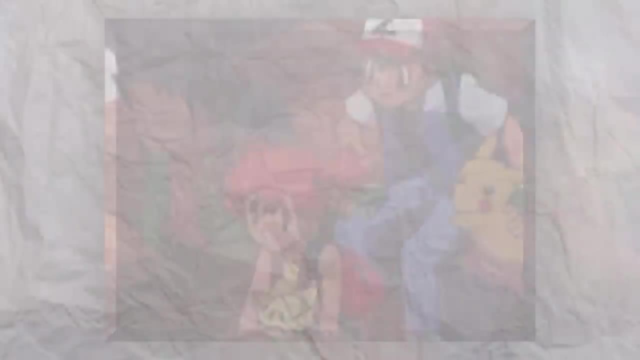 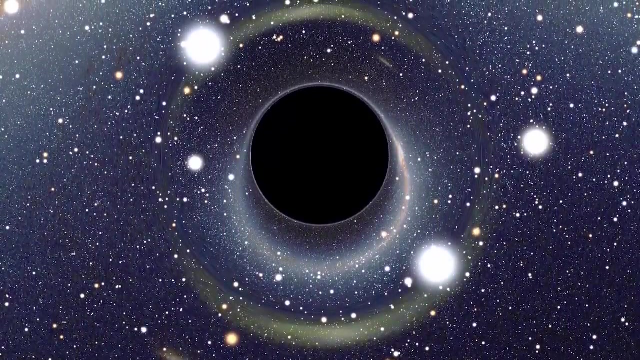 They mostly live in Minnesota. Maybe he really has heard of them. How about PC and Pokeball technology? Well, shoot, If we can just rip holes in time and space. What if these devices use pocket dimensions? What if that's the real reason they're called pocket monsters in the first place? 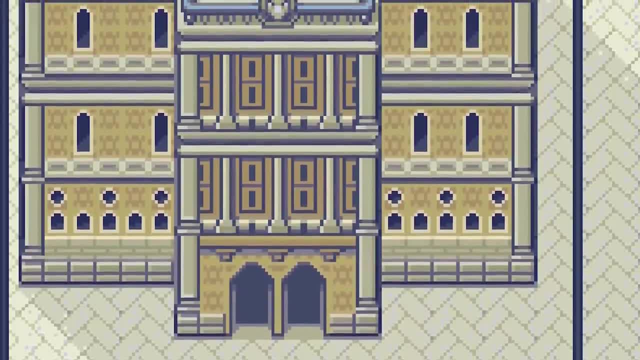 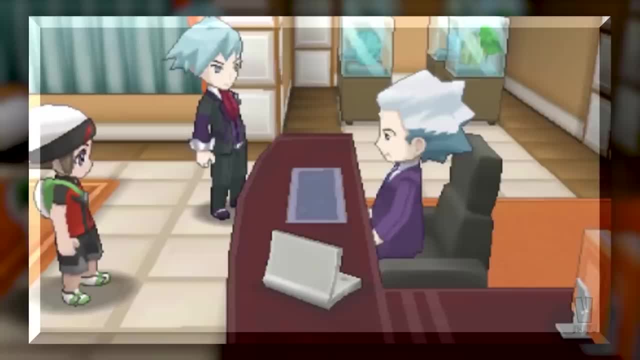 It might even explain Devon Corporation's uncannily creepy new reference for Omanyte and Omastar. Don't tell me you didn't notice all the new symbols hanging around their headquarters these days. Now we know it's literally possible that they visited the Twitch Plays Pokemon universe and learned about Lord Helix himself. 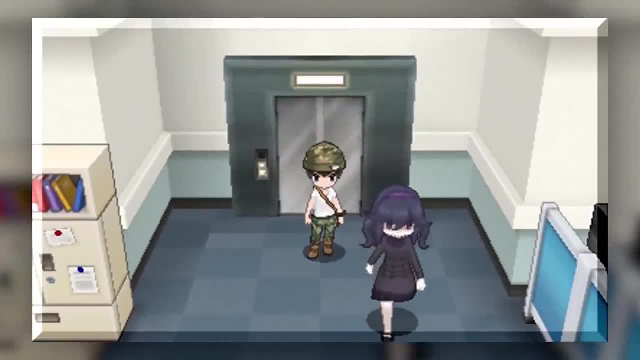 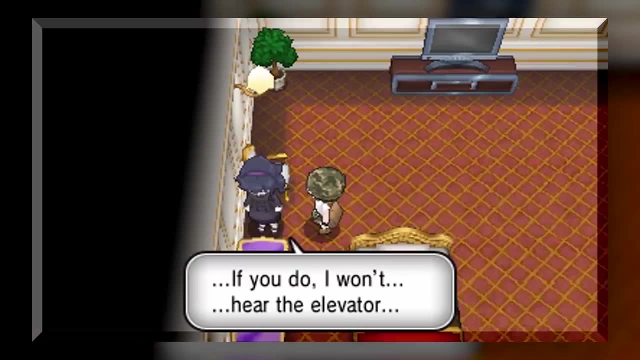 And what about that mysterious ghost girl from Pokemon X and Y who says: You're not the one, You're not the one And then vanishes? We might be witnessing a super creepy rendezvous between two interdimensional travelers. And finally, what if Diglett's mysterious missing feet exist in another dimension? 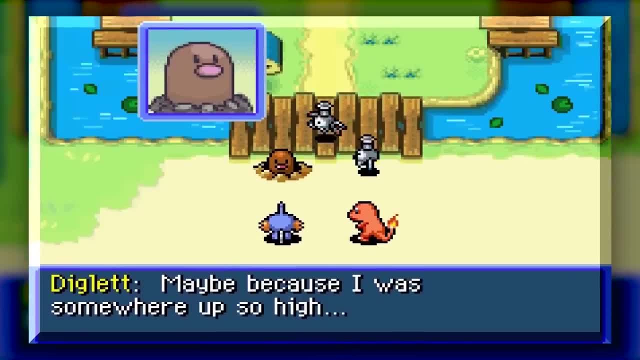 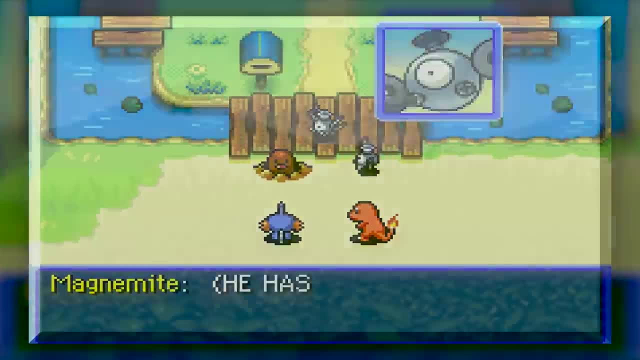 In Pokemon Mystery Dungeon, Red Blue Rescue Team Diglett says his feet feel like they're floating in air. Okay, so maybe I'm getting a bit carried away, But then again, what if I'm not? Maybe Pokemon has always been about other dimensions and the beautiful idea of connecting your little world with someone else's. 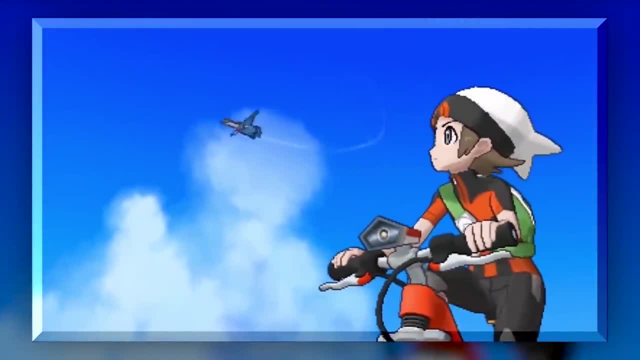 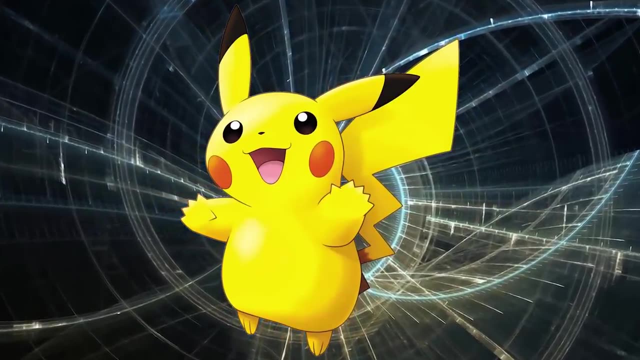 Or maybe it's just something they didn't think about until they realized that fans were asking too many questions. But regardless, who knew that Pikachu would be giving you a little lesson in quantum physics? But hey, that's just a theory, A game theory. 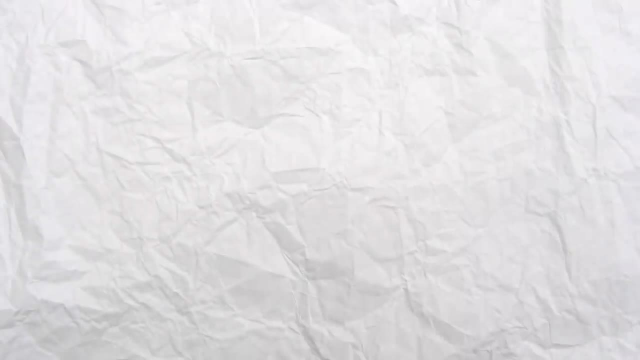 Thanks for watching. Let's cut to the chase. You like snacks? I like snacks. You like free things? I like free things. Get the best of all worlds by clicking the link in the description or typing in natureboxcom slash matpad into the address bar. 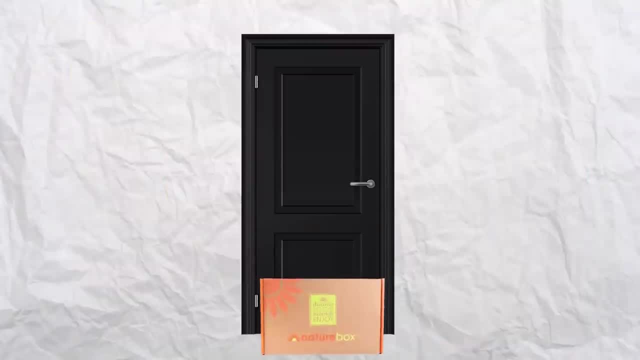 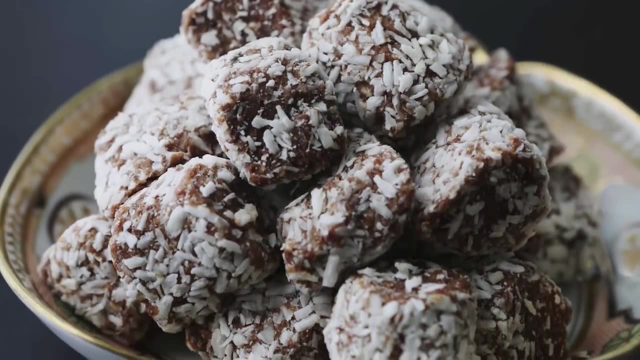 And get yourself some free food sent directly to your door via the NatureBox delivery service. This month I'm dining on chocolate banana chips, coconut date energy bites for those late night game theory sessions, and dark cocoa nom noms, Which are so named because when you eat them, you go nom nom, nom, nom nom. 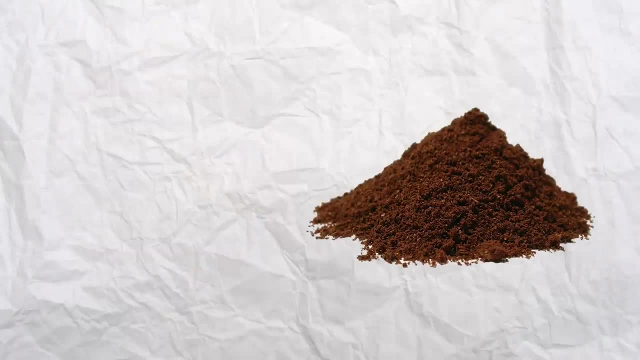 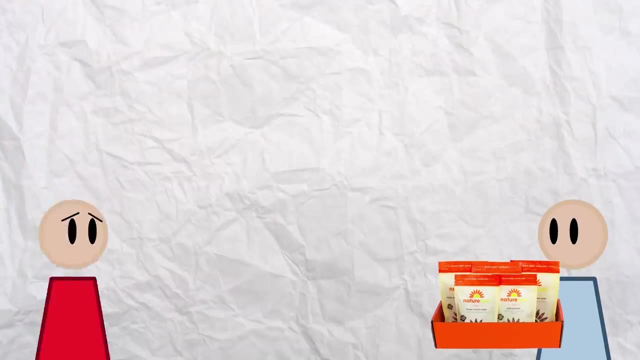 Like Pac-Man, but eating dark cocoa instead of weird white pellet things. Let this be the universe where you get to indulge in some free snacks delivered directly to your door, And let that other universe- you just remain hungry And sad that he didn't click the link in the description.